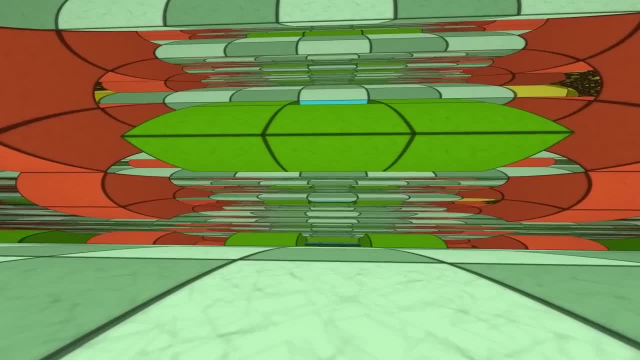 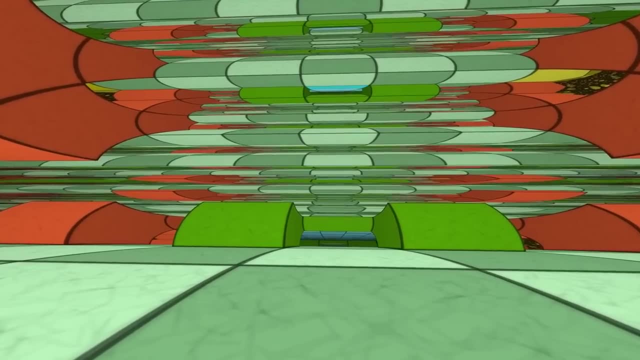 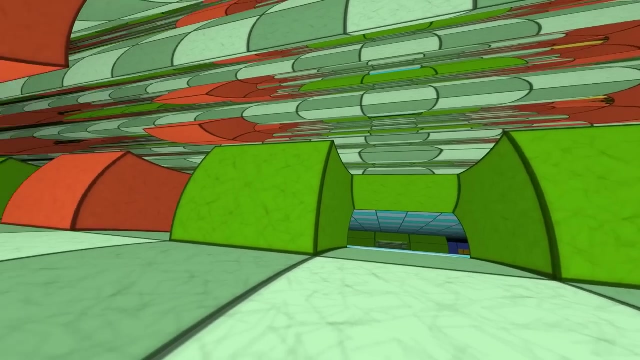 But hey look, As you come closer, this effect becomes weaker. Non-Euclidean geometry comes with perspective working differently than you would expect. Accept that your intuitions gained in the Euclidean world may be useless here. The second rule is pay attention to the shapes you see. 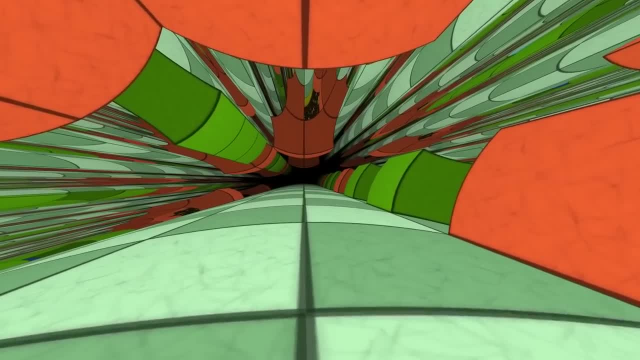 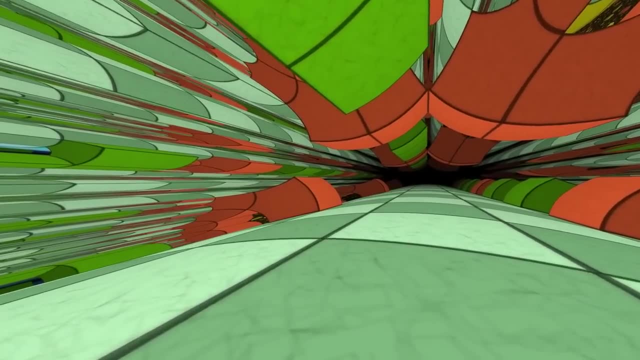 Look, the world is no longer based on the cubes. We told you, this is not Minecraft. The faces we see here are pentagonal. Their edges may appear curved, but they are not. Again, this is only because the perspective works weirdly. 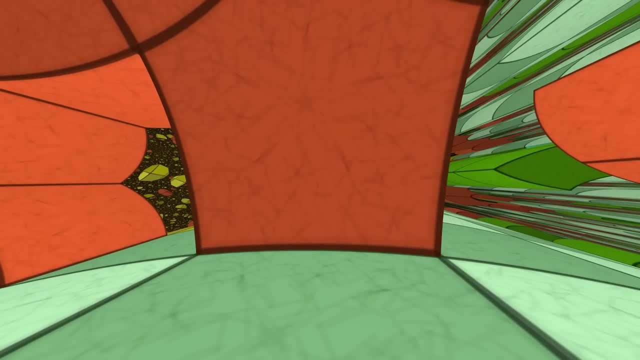 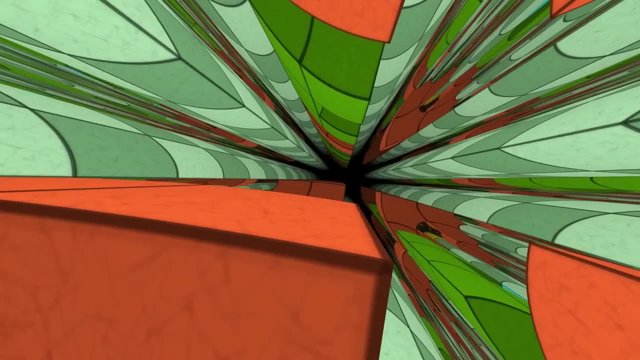 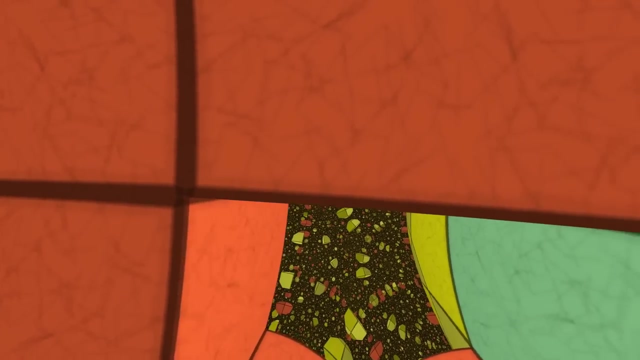 The third rule is: feel free to measure the angles. If you examine any of those pentagons, you will see that the edges are straight. Moreover, all angles of those pentagons are 90 degrees And, yes, this is a shape that is not possible in your Euclidean world. 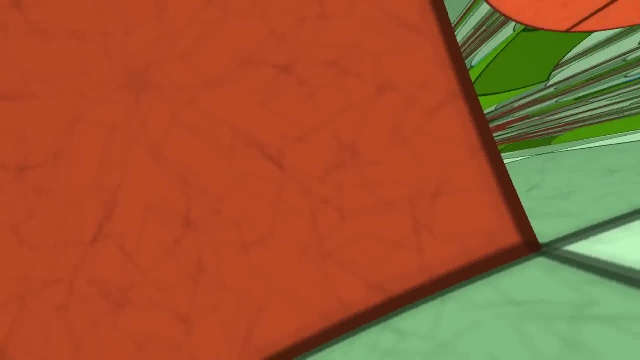 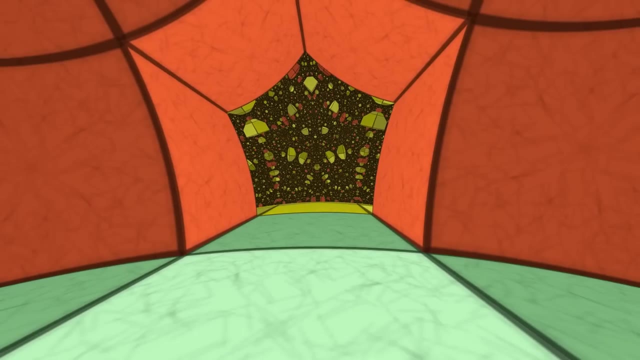 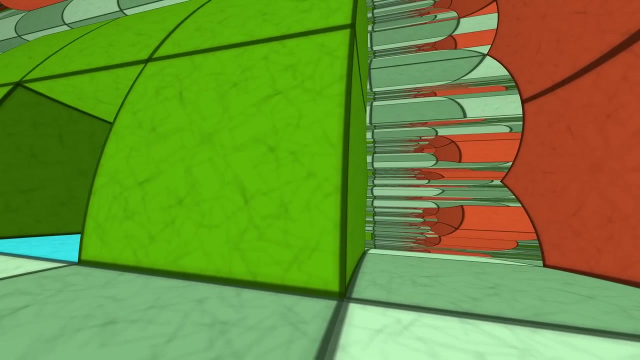 And this is not just a perspective trick. This world is really different. We are now in a hybrid geometry. Even though the pentagons are weird, they are put on each other, just like in the Euclidean geometry. Sidewalls and floors are plain old Euclidean squares. 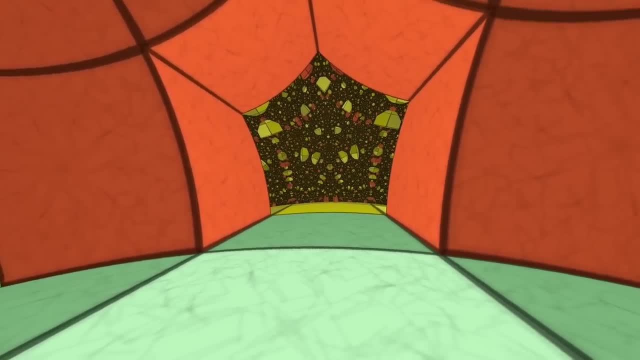 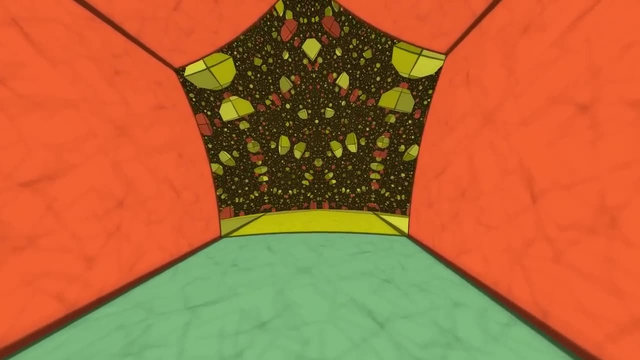 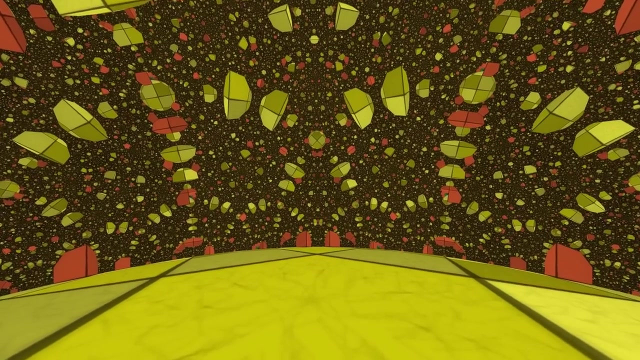 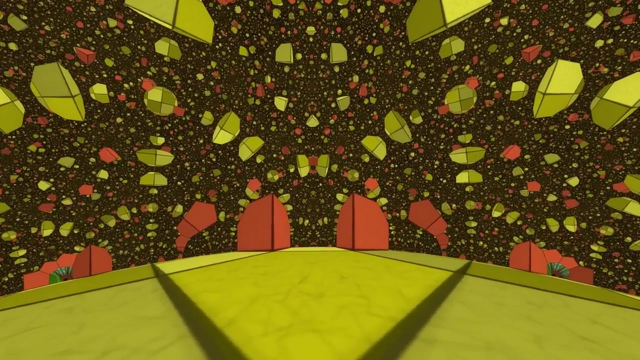 Okay, let's use another portal to understand where the weird pentagons come from. Welcome to three-dimensional hyperlinks. We are now in a hyperbolic geometry, the homeland of the weird pentagons. Now you see them everywhere, just like you saw squares everywhere in the starting Euclidean world. 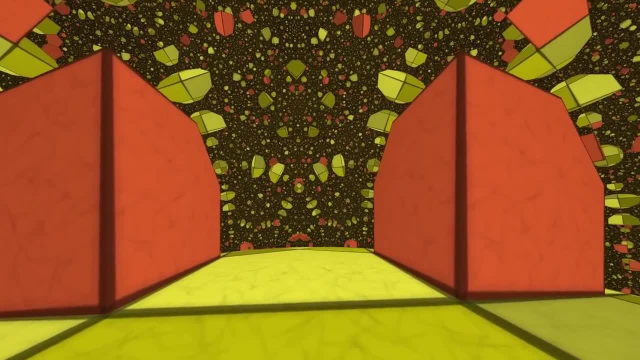 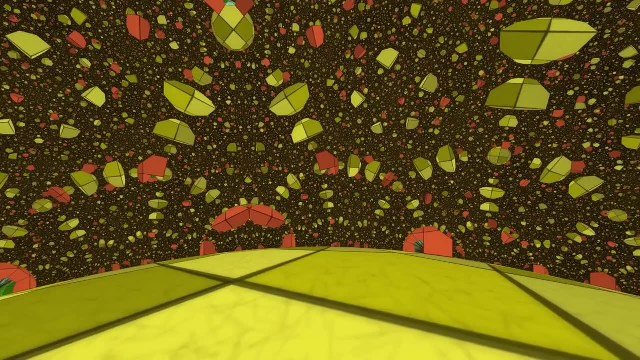 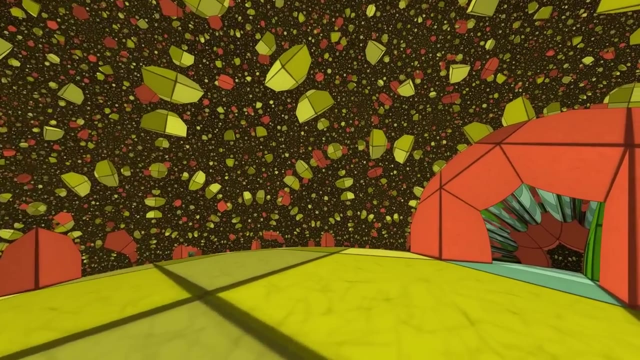 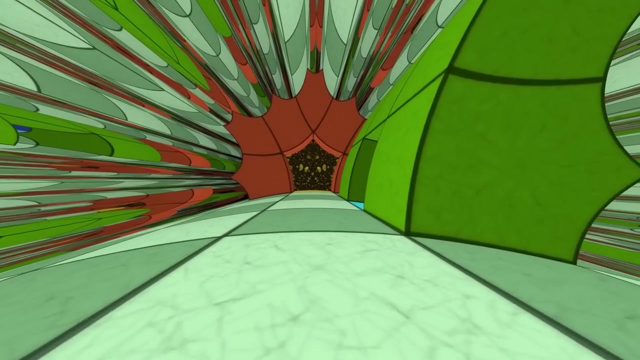 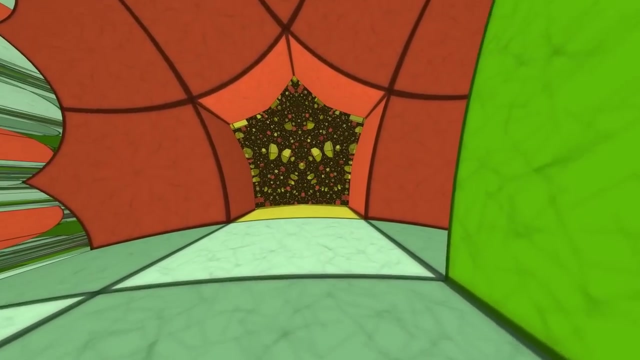 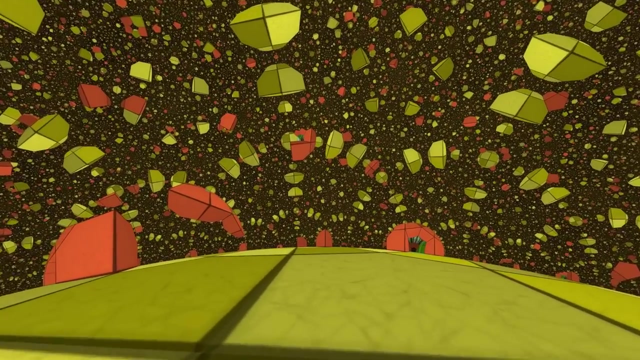 This is not a hybrid geometry, so the perspective effects are more consistent. Now you see clearly that the edges are straight. Even though there are no stretching effects, the perspective is still not what you would expect. The kita is not blended in one way. there is no. wedge in this plant And although腐 väldigt først نlove tył し blob, most often It feels more like fast zooming in than moving forward, which is especially visible when you enter the portal. We didn't want to scare you, so we slowed you down. 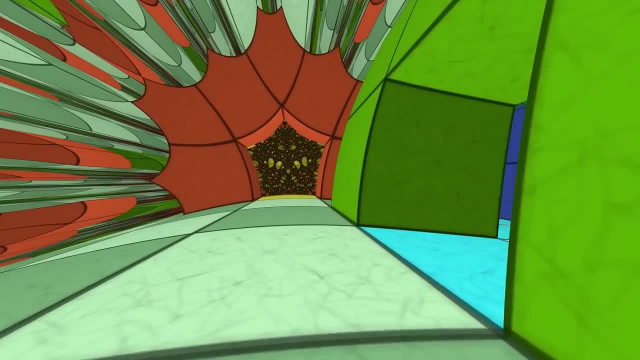 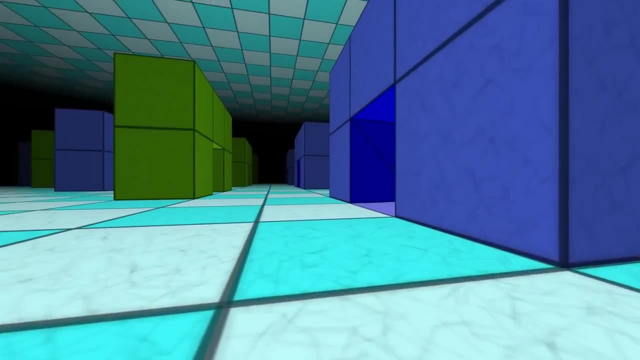 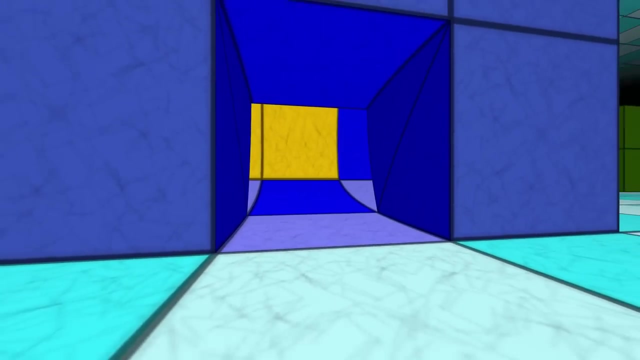 Now let's cross the portal again, but at the normal pace. enough, you might need some rest in the Euclidean world. Just joking. the hyperbolic geometry is not the limit. Our tool will take you through even weirder geometries. 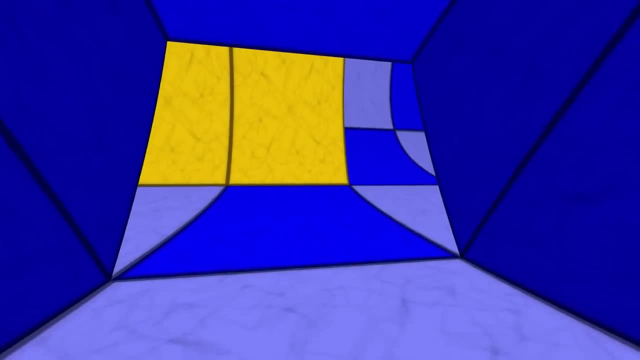 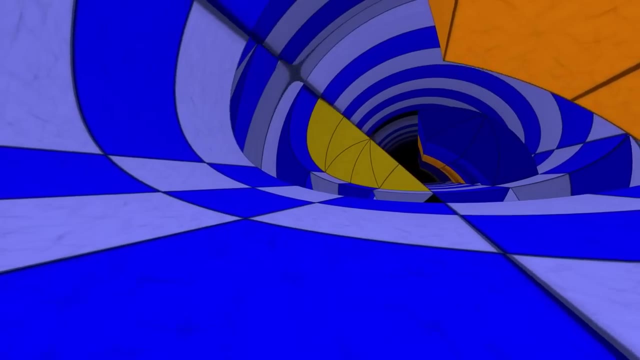 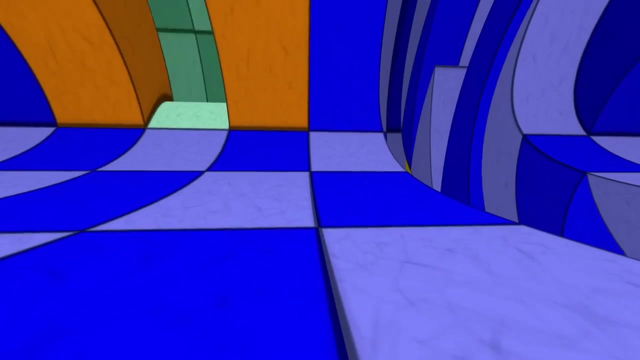 Look, here is another portal. This is another hybrid geometry. Previously we stacked weird pentagonal objects from the hyperbolic geometry. Now we stack spheres. Ok, ok, yes, this might surprise you. We know you imagine spheres to look differently and that you even live on a surface of one. 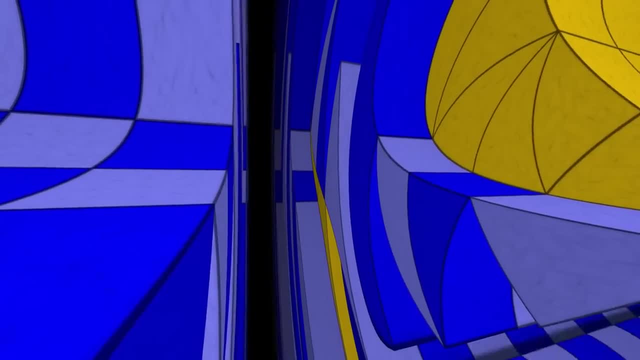 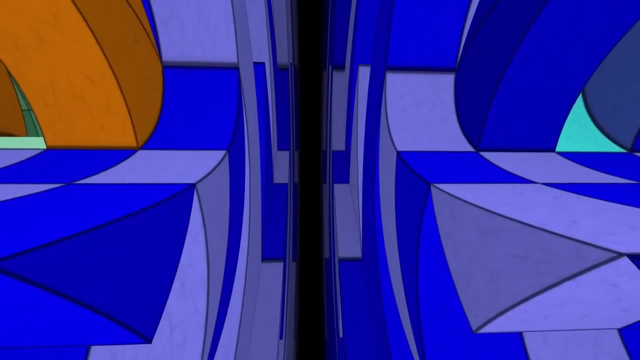 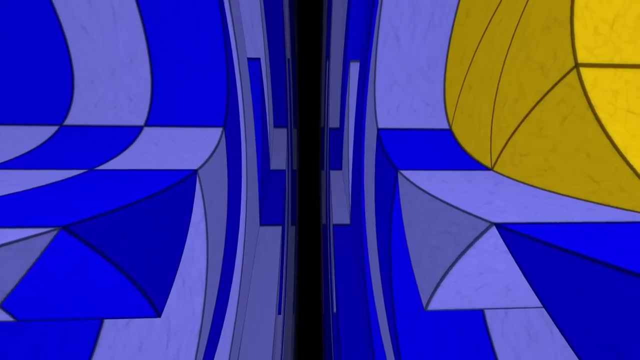 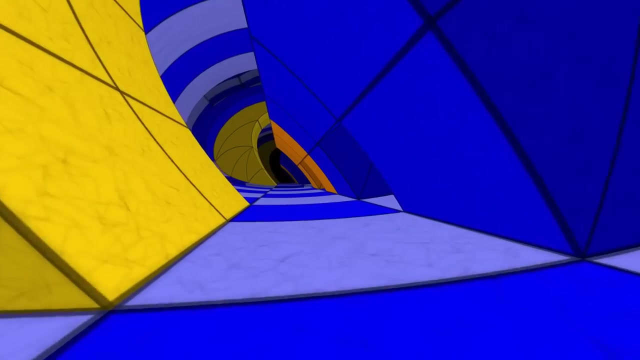 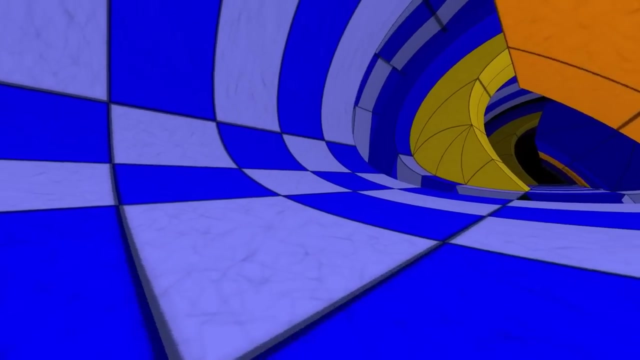 Sorry, deal with it. For your convenience, we have equipped you with jetpacks. Hope you enjoy the view. The spherical geometry is the opposite of the hyperbolic geometry. Note that the objects far away are stretched vertically. Recall, they were compressed in the previous hybrid geometry. 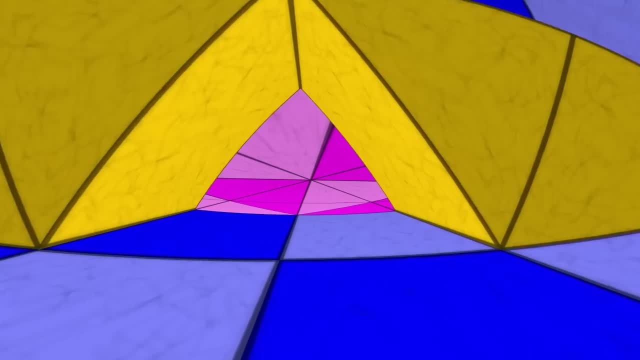 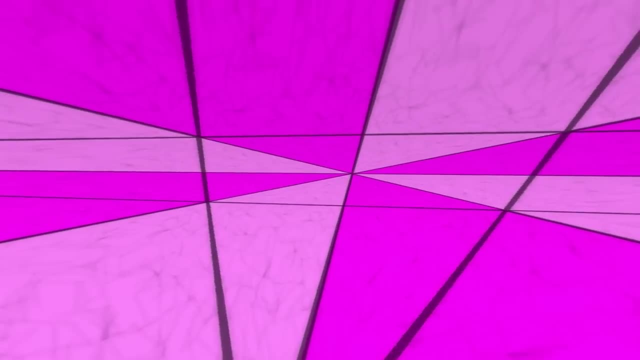 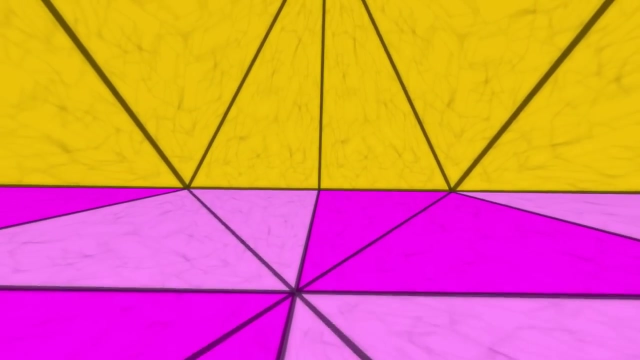 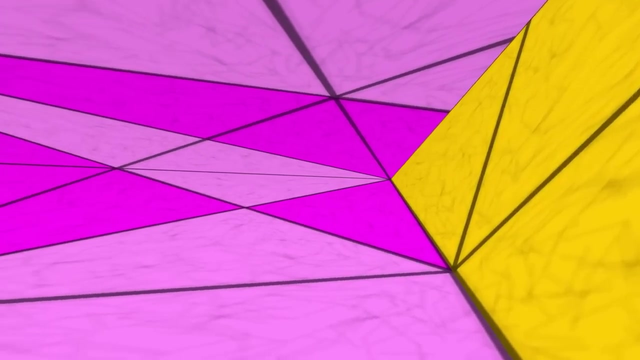 Time to enter spherical geometry. There are no parallel lines here. They always cross. This is a very, very small world. Not much to explore here. Let's go back In the spherical geometry. objects that are far away from us appear to be relatively big. 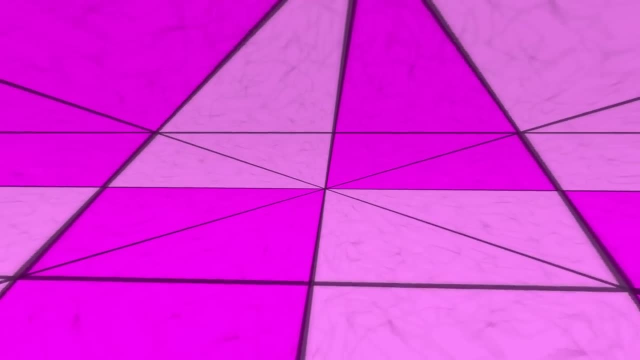 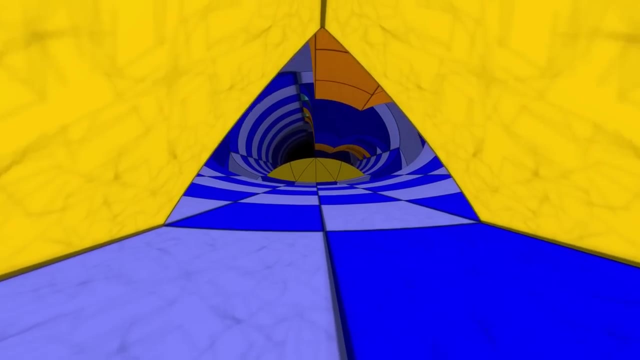 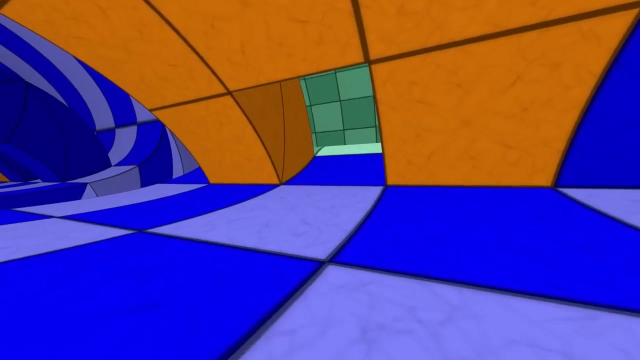 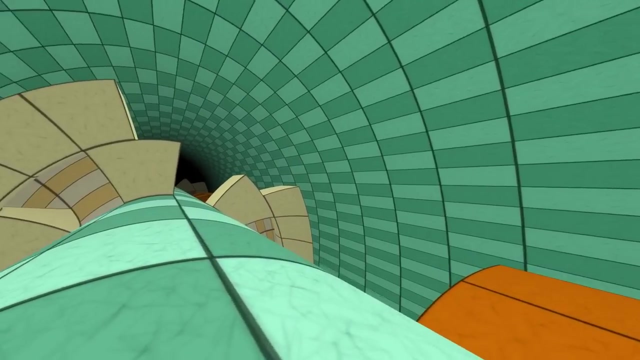 Look at the portal here. As we are approaching it, it becomes smaller and smaller to us. Ok, Ok, Let's dive in. Oh, another portal, Let's dive in. Do you know where we are? This is again hybrid hyperbolic geometry.